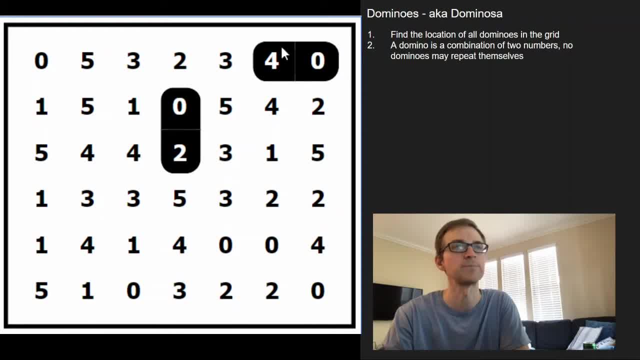 then repeat themselves. So that would force it to be a zero four, And what you're looking for is all of the instances. So in a five by five grid you're going to go all the way up to the fifth digit. So zero, zero, zero. one, zero, two, zero, three, zero, four, zero. 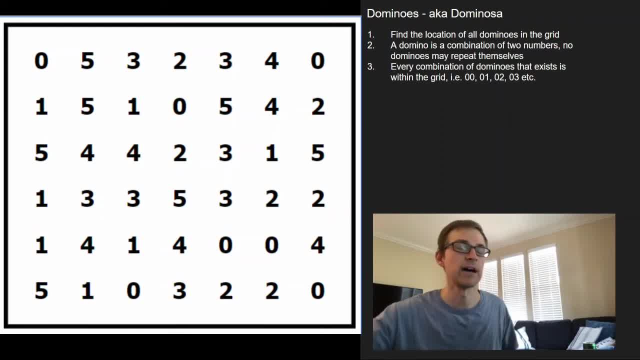 five, and then one, one, one, two, one three, one four. So you're going to go all the way up to the fifth digit. So zero, zero, zero, one, zero, two, zero, three, zero, four, zero one, five, and so forth. So that's it for the rules, What I'm going to go ahead and 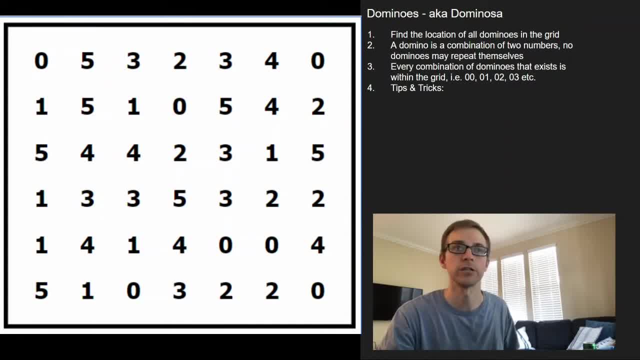 do is try to solve this puzzle for you guys and share some common tips or tricks that will hopefully make it easier for you to solve them yourself in the future. So the good place to start is going to be the corners, And what you're looking for is any repeating instances. 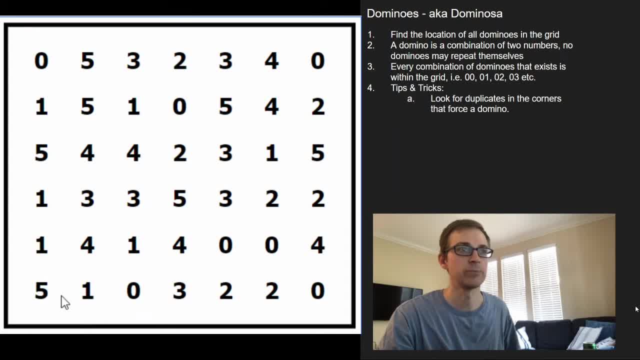 So this one five, for instance, is repeated. So, no matter what, if the domino looks like that or like that, you have a one five combination. So that makes it so that there can't be any other one five on the grid, right? So we know. 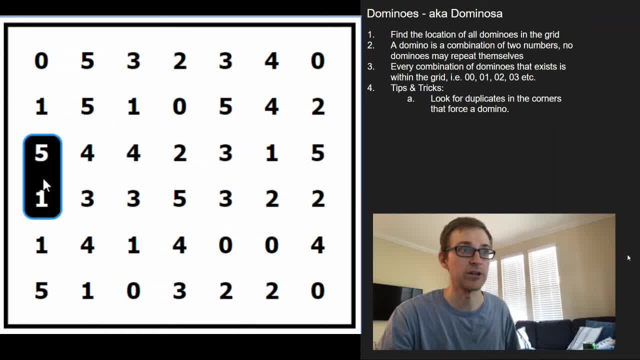 that this can't be a domino, that can't be a domino, and that can't be a domino because there's already a one five in the grid. So how this is helpful is you could then draw a line or wall off, knowing that this cannot exist. And same thing there. 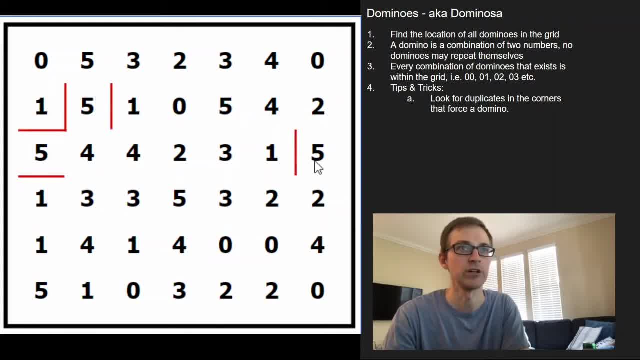 And you can see what this has done: drawing a line between all the ones and fives. is it forced, this domino to exist, this zero one, because this one can't go anywhere else but up? So that is helpful, because now we can repeat the process of drawing a line between: 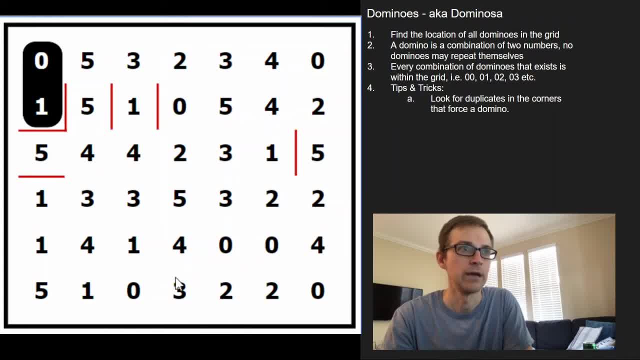 all the zeros and the ones And like that, And that's forced another domino. So this zero now has to come to the right And we repeat the process again, drawing a line between any of the zeros and threes. I think that's it. 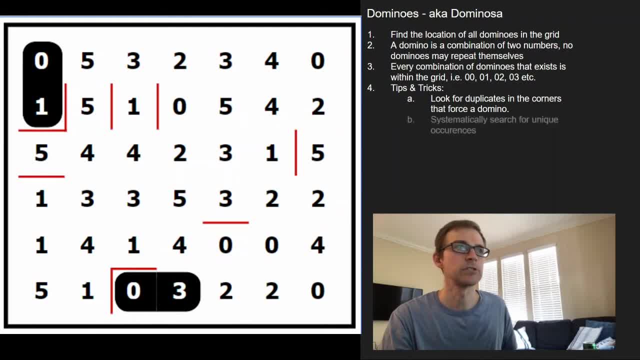 The next thing that I would say is, after looking at the corners, is: look for any unique dominoes that exist, And I do that in a systematic way so that I don't miss anything. So I first start with the zeros, And what we're looking for is unique instances, right? So this zero. 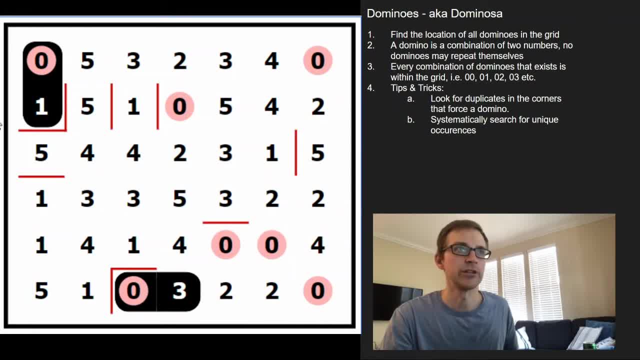 zero. that's the only zero, zero domino on the grid that can exist. So we know that that's a domino, Right? If let's say, see if I can come up with another example. So let's if we look at the ones. 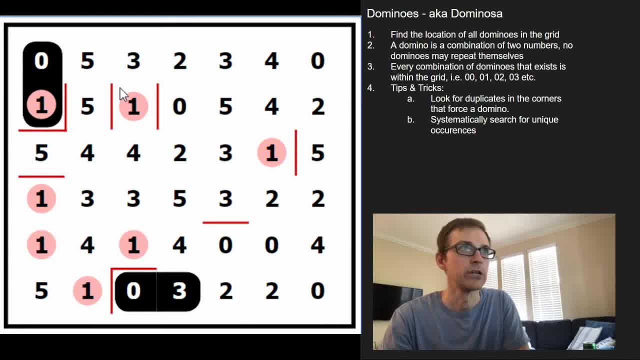 there's many one, four combinations, So we don't know if it's a one, four like that or like that. So that would not be helpful. Whereas the zeros: we know that that must be the domino And what that's done is that's forced. then this two, two and this zero four. 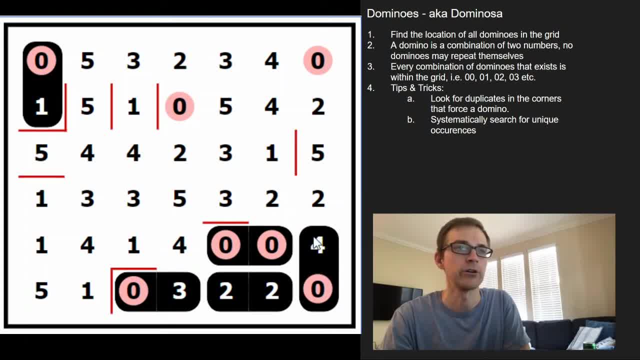 And then we have this two, two and this zero four, And then we have this two, two and this zero four, And we can do that earlier trick where we have to block off these twos because we know that they can't repeat, So we can draw a line there, And then, with the zero fours, we can draw lines And 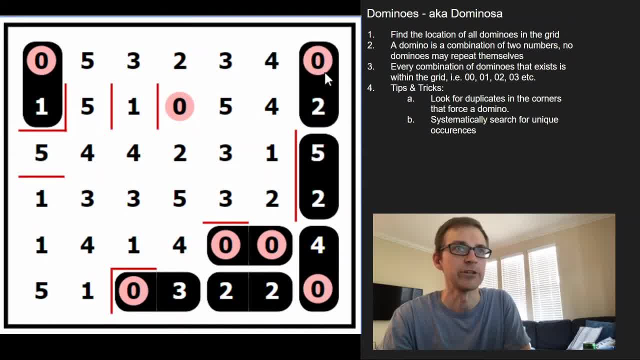 that's helpful, because that's going to now force some more dominoes. Oops, like, just like that. So now we can't have any two fives repeat. So draw a line between those two fives, That's it. So there's a domino here that's forced this five, four. That forces this five, five, oops. 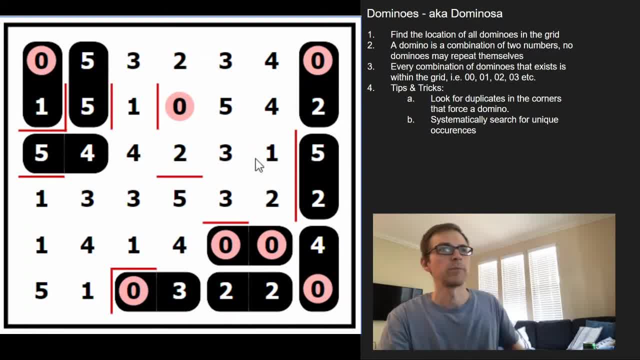 And we're making progress. So the next thing I'd say is that as you go along, you're going to be creating new corners constantly, And so you can use that first tip time and time again. So you can see, now this four is a new corner And this two is a new corner. 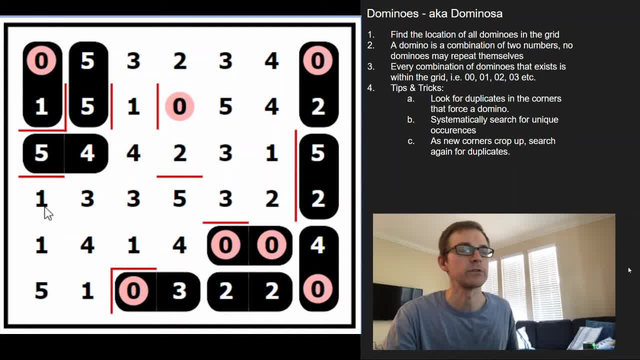 this 3 is a new corner, so you could use that first trick time and time again and I would definitely recommend that is that's going to be helpful for you. another thing is: in the harder puzzles you want to remember that dominoes always have to have an even number of digits so you can never have a closed. 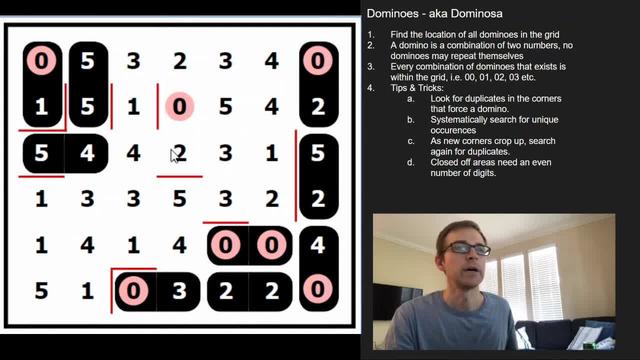 off area with an odd number. so what I mean by that is if let's say, for instance, see if I can do an example here- if I did this domino that closes off this region, now this is okay because there's six digits in here, but if, on the 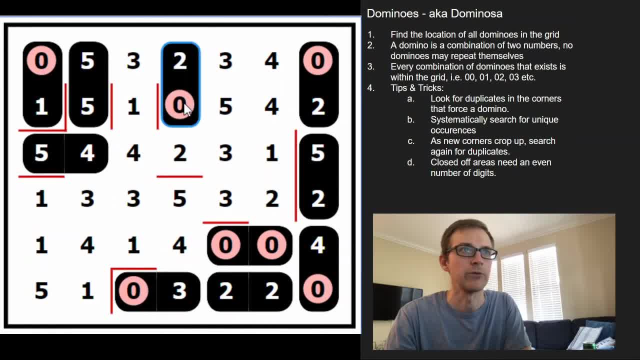 other hand, I don't know we closed off an area like this. this would not work, because now you have an odd number of digits, so hopefully that makes sense. and then the other thing is, if you have an odd number of digits, you can never have an odd number of digits, so hopefully that makes sense. and then 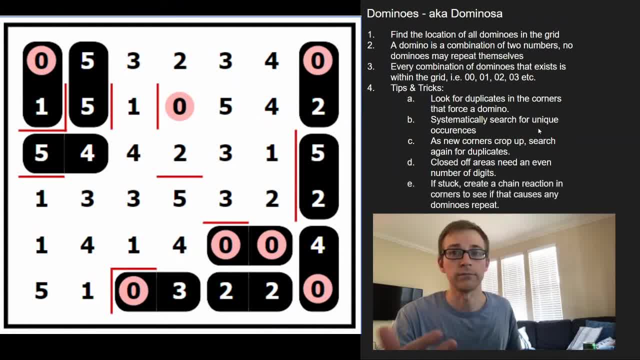 the last thing I would say is: if you're stuck and you're not got, you just don't know what to do. it's a hard puzzle. you can artificially create chain reactions to see if there's any illegitimate dominoes. what I mean by that is if we 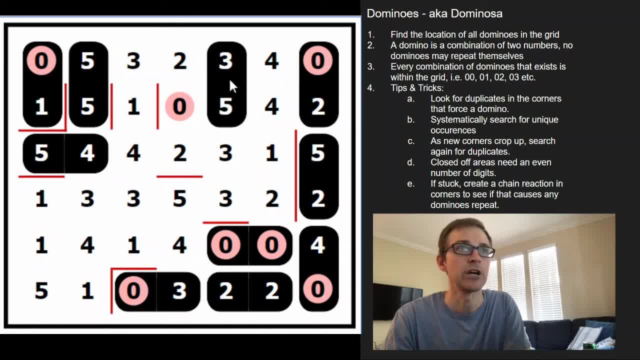 were to say, put a domino here, that would force this 4, 4, and that's okay, so that doesn't help us. but let's say, for instance, we created a chain reaction like this with this: oops, sorry, this 3, 3, that would 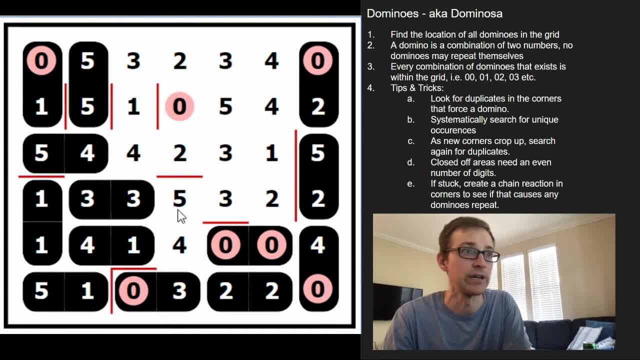 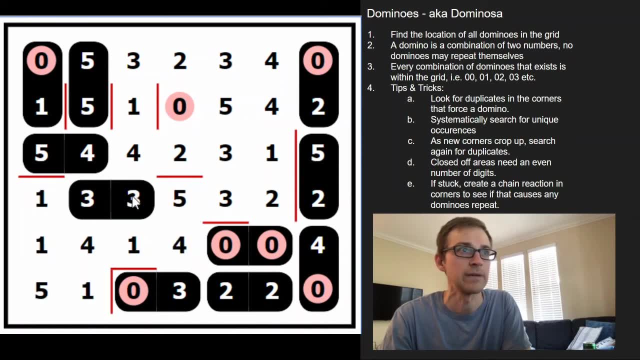 force this 1 1, force this 5, 1, 4, 1, 5, 4 and it would create all of those dominoes and we would look to see if any of those dominoes are illegitimate. and if they are, then we would know right from the get-go that this 3, 3 is not a domino. it's rare. 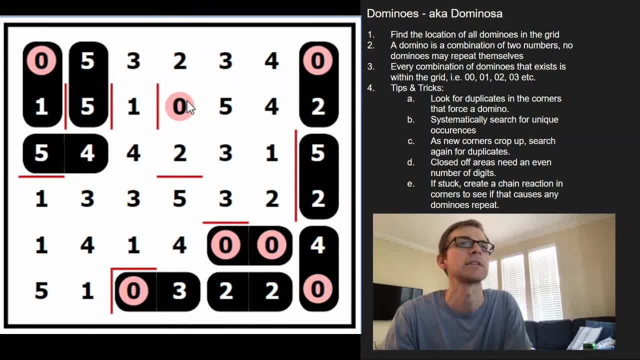 that you'd have to use that tactic again. you would typically only use that tactic in a very hard dominoes puzzle or if you're stuck and you can't find any unique circumstances. so hopefully that's helpful. I think from here I can finish this puzzle off fairly easily. we're looking